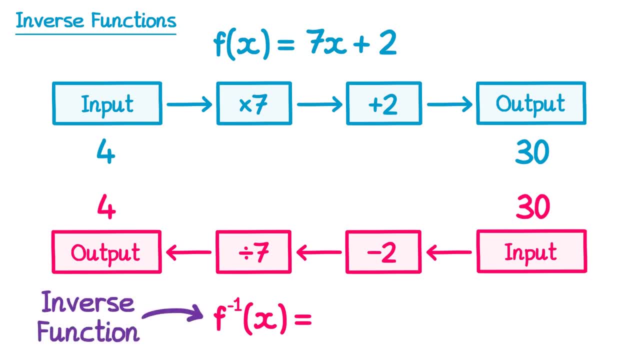 with a negative 1.. This simply means the inverse function. You shouldn't confuse that negative 1 with a power negative 1.. It doesn't actually act as a number in this scenario. it's just the way we write an inverse function. So if you ever see f with a negative 1 there of x, this just means 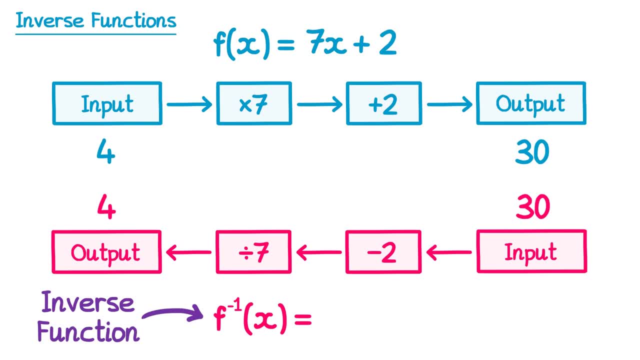 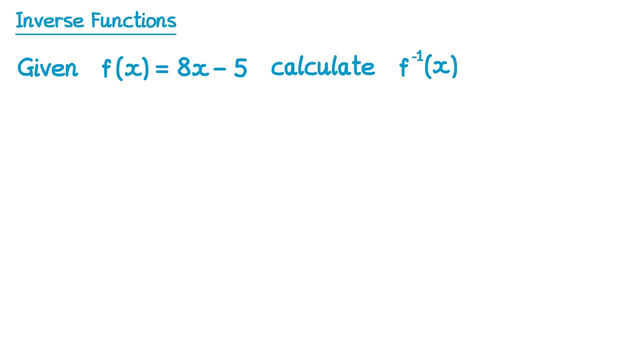 inverse f of x And we actually just worked out this function. So we subtracted 2 and then we divided by 7.. So we could say inverse f of x equals x minus 2 and then divide by 7.. In your exam you may be given a function and asked to work out its inverse. 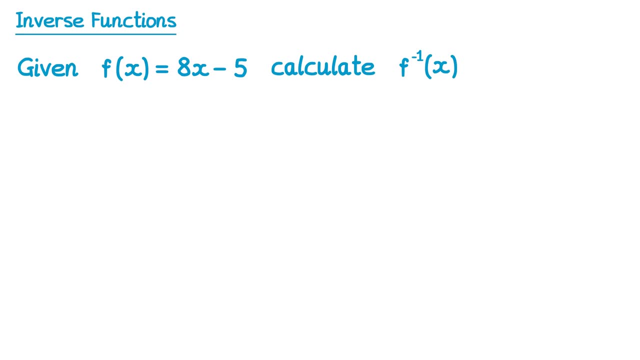 There is a method that works well for this. it means you don't have to draw out those function machines each time. The first step is to write out the function and change the f of x for a y. So the function here is: f of x equals 8x minus 5, but I'm going to replace the f of x with a y. 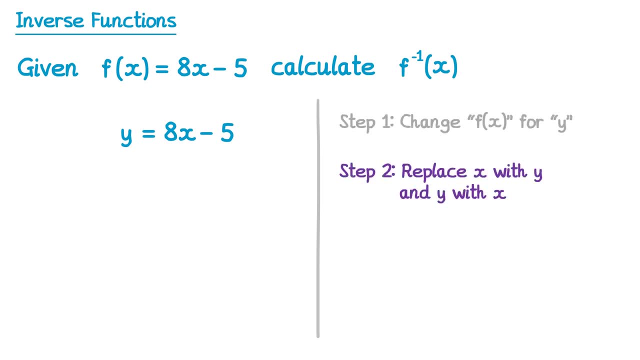 Then onto step 2.. So step 2 is to replace the x with a y and a y with an x, And this applies to all y's and x's that are in your function. So if you have many x's, all of the x's turn into y's. 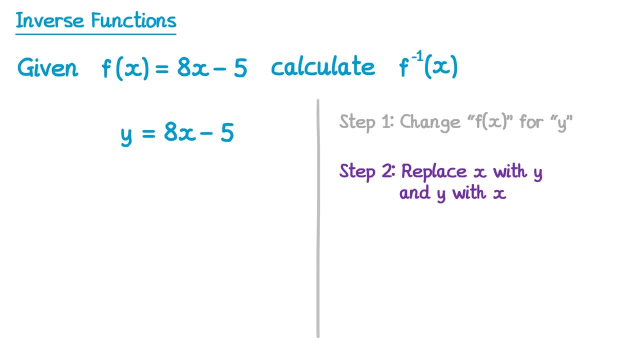 and any y's turn into x's. In this case we've just got one of each, so I'm going to replace that y with an x, so it's x equals, and then replace the x with a y, so it's 8y minus 5.. 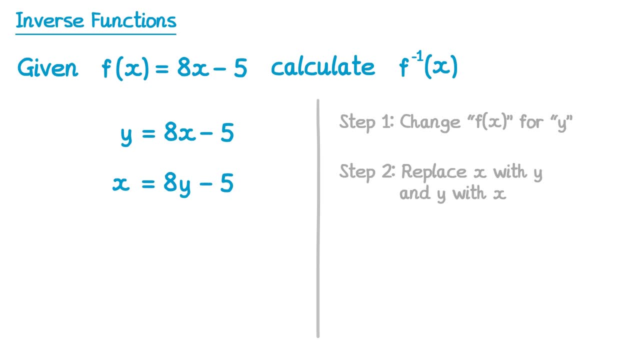 And that's step 2 complete. Then we move on to step 3, which is to make y the answer for x subject. so we need to do a bit of rearranging. First of all, I'm going to add 5 to both sides. 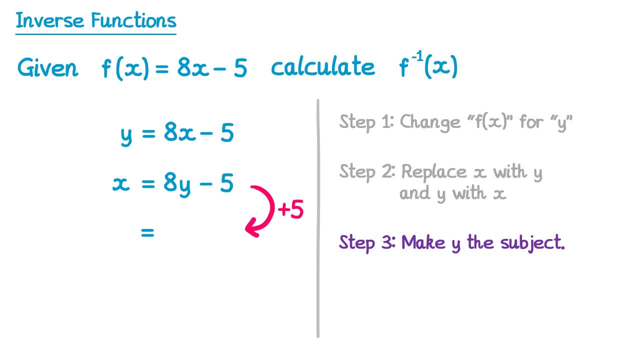 If I add 5 to the right hand side, that'll cancel the negative 5 that's there and leave me with 8y. and if I add 5 to the right hand side, well, there's already an x there, so I just need to add 5 to. 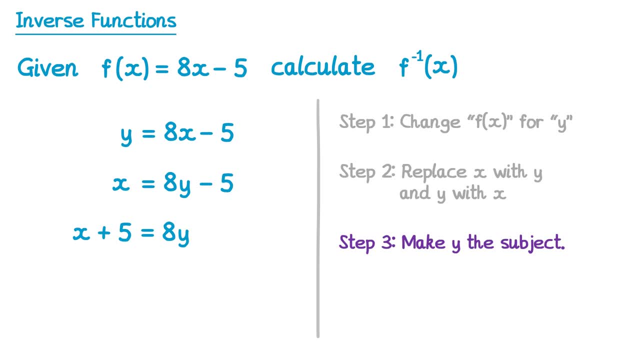 that. so that's x plus 5.. We've got one more step to go. on the right hand side I've got 8y. so if I divide both sides by 8, on the right hand side 8y divided by 8 is just 1y, and on the left hand 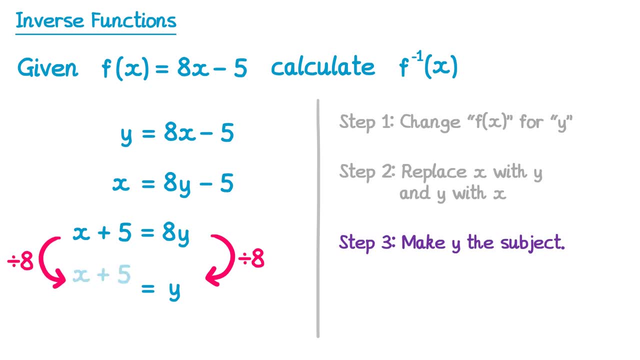 side. I've got x plus 5 and I divide that by 8, that's x plus 5 divided by 8.. So step 3 is complete onto the final step. Step 4 is to change the y into inverse f of x, so we can just remove that y. 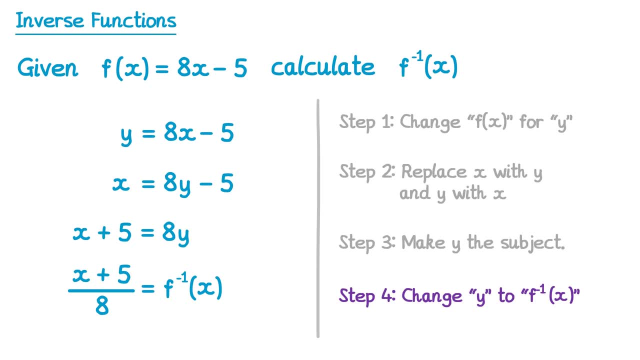 and replace it with inverse f of x. and normally when we write functions we'd write the function bit on the left hand side, so we can just switch those last two parts around and here's the answer. so the inverse function is x plus 5 over 8.. 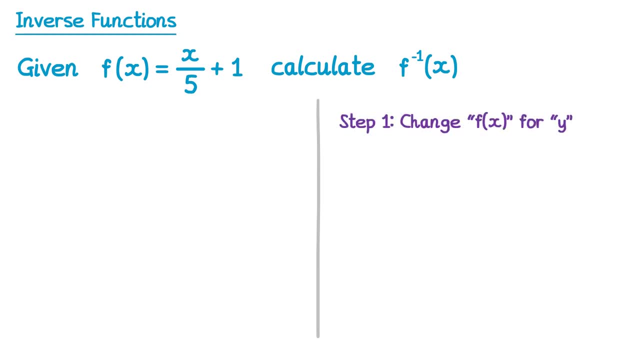 Let's try this one. So we're going to go through the same steps. we're going to change f of x into y first, so let's replace the f of x with a y, and then onto step 2. we're going to change all of the x's. 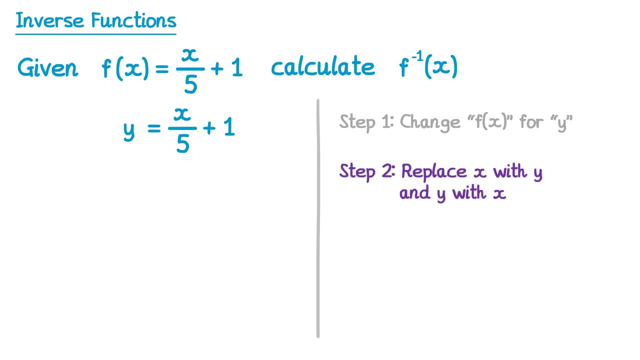 with y's and all of the y's with x's. so instead of y equals at the beginning is x equals, and then, instead of x over 5, it's y over 5, and then plus 1, and then onto step 3, which was rearranged to make. 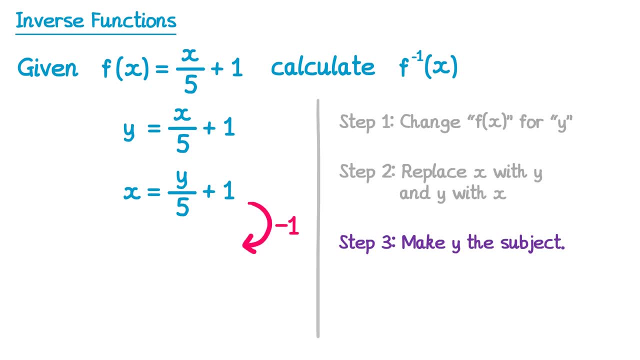 y the subject. so for this one I'd subtract 1 from both sides. if we do that, on the right hand side we get y plus 5.. over 5 the 1s will cancel. and on the left hand side, if we subtract 1, it's x. take away 1. 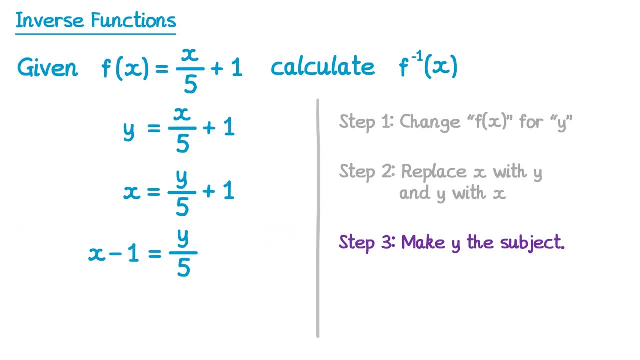 and then I have y over 5, so I can multiply by 5 on both sides. On the right hand side this will cancel the 5 to give me just y, and on the left hand side I've got x minus 1 there and I need. 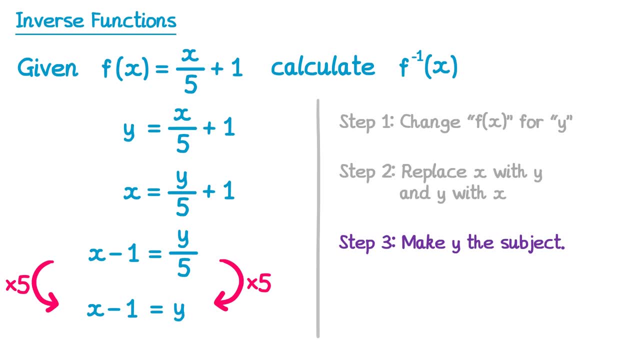 to multiply this all by 5.. The best way to do this would be to put it inside a bracket and then multiply by 5.. So onto the final step. we can just replace that y with the inverse function of x and then switch the order around, and there's your answer. If you wish, you could expand that bracket. 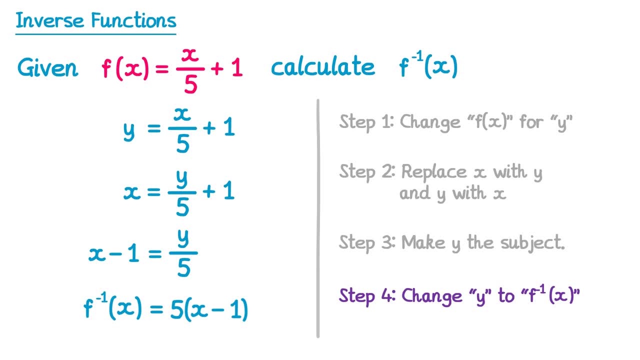 to get 5x minus 5, but it wouldn't matter. this would still be fine as your answer to the inverse function. Now let's try another one. we're going to do exactly the same steps, so change f of x for a y, so instead of f of x equals, it's y equals. then onto step two. 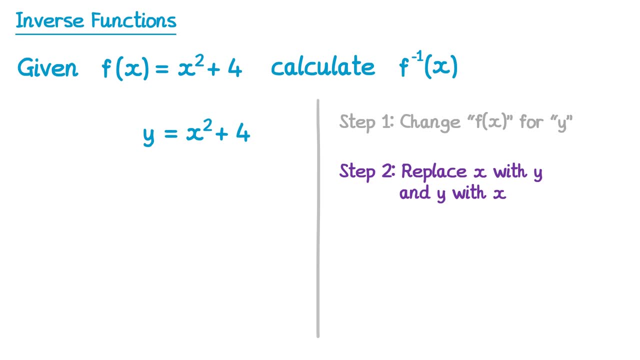 Which is, replace all of the x's with y's and y's with x. so instead of y equals it's x equals, and instead of x squared it's y squared, and then plus 4.. Now we move on to step three. let's rearrange to make y the subject, so let's subtract 4 from both sides. If you do this on the right. 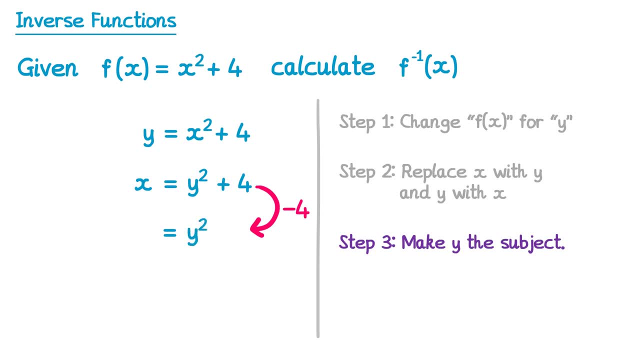 hand side, that'll cancel the 4, to leave you with y squared. and on the left hand side, if you do x take away 4, that's just x take away 4.. Now we're trying to make y the subject and we've got y. 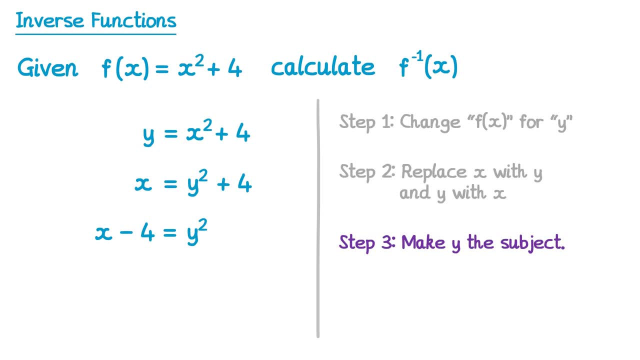 squared. so to undo that squared, we're going to do x, take away 4.. Now we're trying to make y the subject and we need to square root both sides. So if we square root the right hand side, you'll end up with y, but when you square root the left hand side, you end up with the square root of x minus 4.. 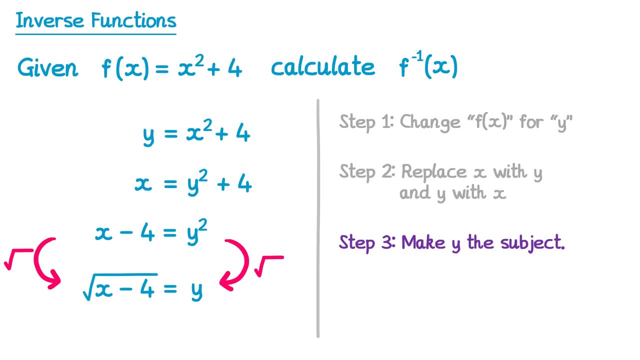 Now, you'd be correct here to point out that when you square root both sides of an equation, you need to consider both the positive and negative root, so we could write plus or minus. However, when we're writing a function, we would never do this. This is something you touch on. 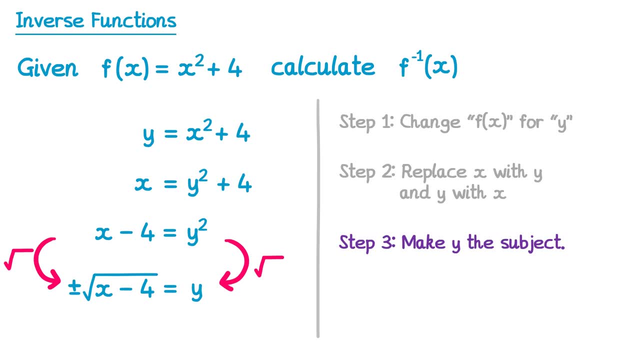 more at A-Level Maths, but a function needs to be well defined. This means that for each of the inputs there can only be one output, and in this case we're going to write a function that's with the plus or minus for each input of x. you'd have multiple outputs, So we just take the. 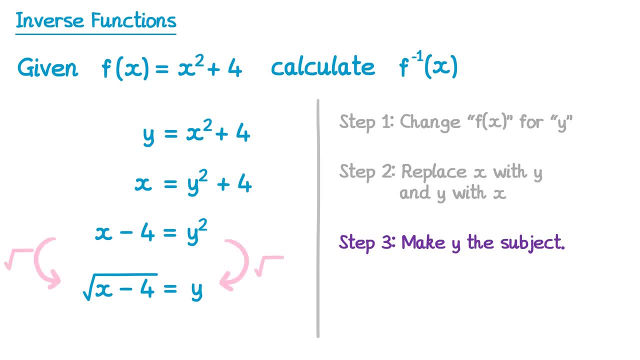 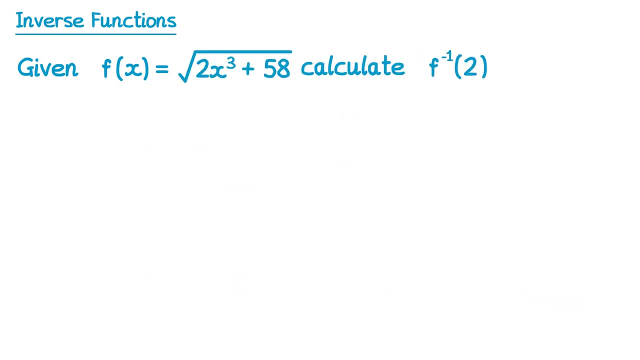 positive one, in which case we don't write plus or minus at all. So on to the final step, step 4.. Let's replace that y with f, inverse of x, and then we'll just switch that around. so the inverse function is the square root of x minus 4.. Now, sometimes in exams you get a question that looks: 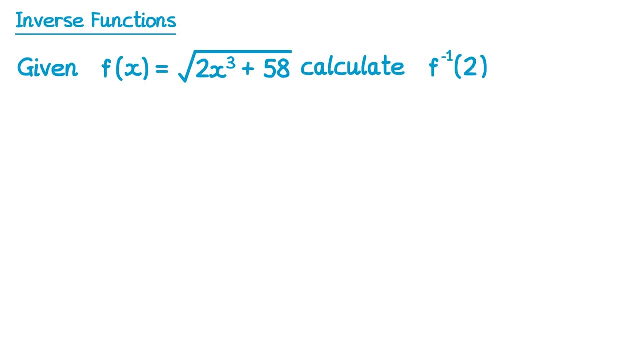 like this. We haven't been asked to find inverse f of x, but instead inverse f of 2.. To do this, we're first of all going to find the inverse function. So let's repeat those steps in the same way. Let's write out the function, but replace the f of x with a y. Then we're going to. 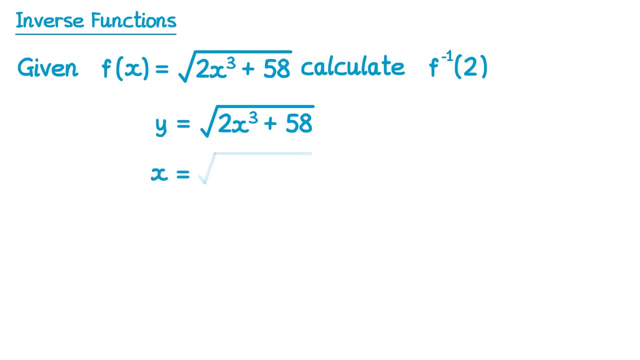 swap all the y's and x's, so it's x equals the square root of 2y cubed plus 58, and then we'll rearrange to make y the subject. So for this one we have a square root on the right hand side. so 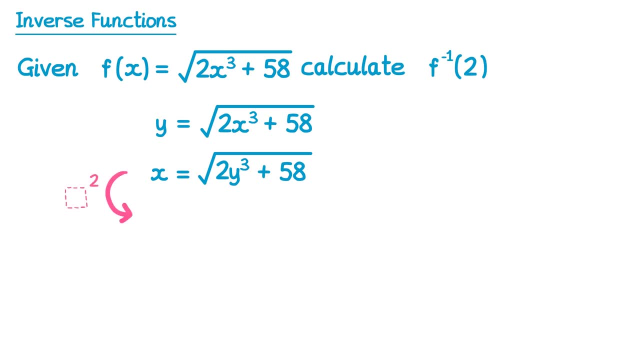 the first step is to square both sides. If we square the left hand side, we get x squared, and if we square the right hand side, that would be the square root of 2y cubed plus 58.. So that's all removed the square root. so we just get 2y cubed plus 58.. The next step is to take away 58. 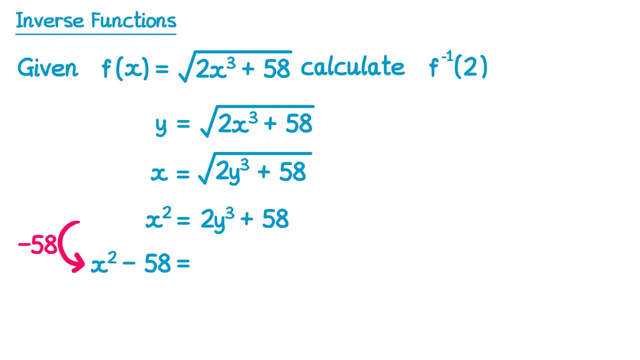 from both sides. If you take it from the left, it's just x squared minus 58, and if you take it from the right, that will cancel the 58 and leave you with 2y cubed. Now we can divide both sides by 2.. 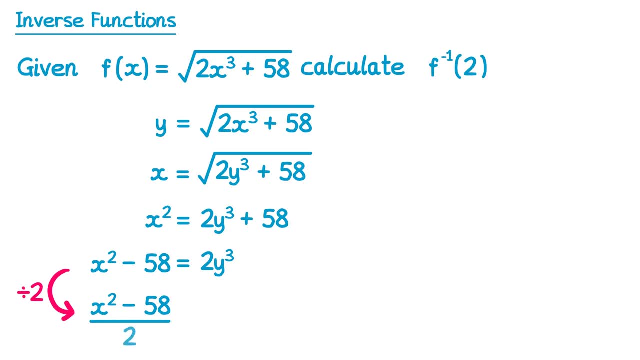 On the left hand side that's just x squared minus 58 divided by 2, and on the right hand side that will cancel the 2, leaving you with y cubed. There's one more step of rearrangement to do So. we've got y cubed on the right hand side and on the left hand side that will cancel the 2.. 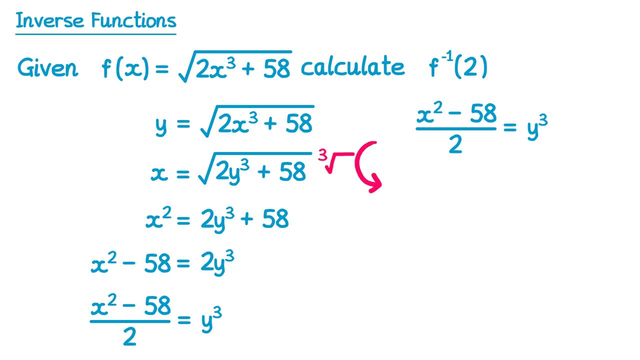 So we're going to cube root both sides. If you do that, on the left hand side you'll get the cube root of x squared minus 58 over 2, and on the right hand side, if we cube root that, we end up with y. 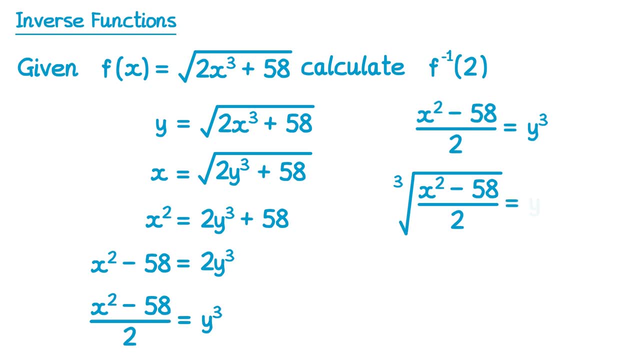 We can replace y with f inverse of x and switch the order around and there's our inverse function. Now remember, we didn't want to find the inverse function, we wanted to find the value of it when x equals 2.. So all we do to find f inverse of 2 is write this function out. 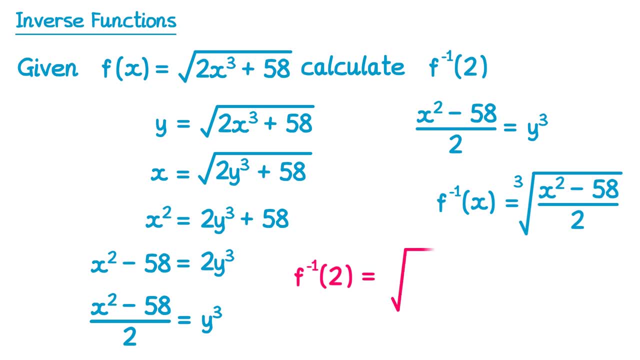 and replace the x's with 2.. So it's the cube root of x squared. but we know that x is 2, so 2 squared minus 58 over 2.. 2 squared is just 4, and 4 take away 58 is negative 54, and if you divide that by: 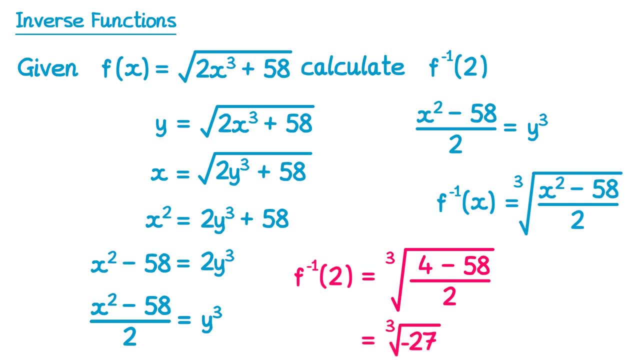 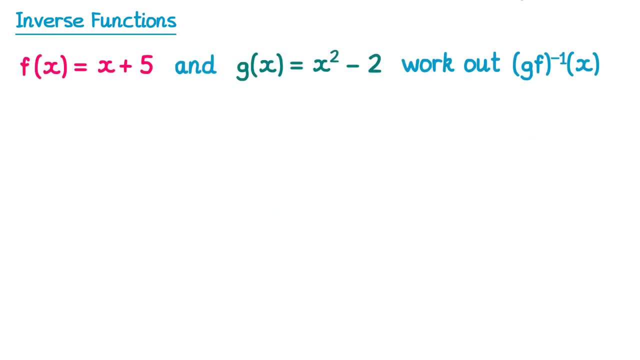 2, you get negative 27.. So it's the cube root of negative 27 which is negative 3, and that's your answer to this question. And now let's look at one more question for this video. In a previous video I looked at composite functions, and this is a great topic to be. 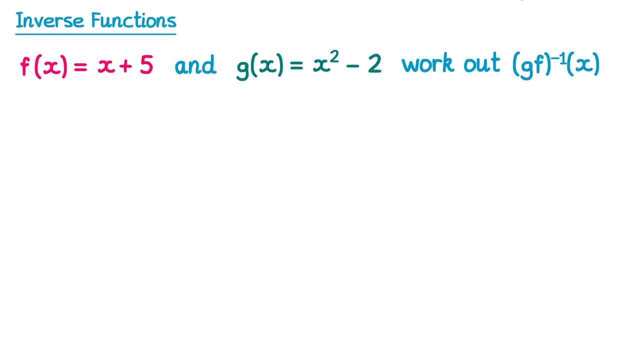 mixed with inverse functions. Often in exams you'll get functions questions which assess multiple different skills in one go. So in this question we've been asked to find g f- inverse of x. This means we need to do the composite function g f of x first and then find the inverse of that. 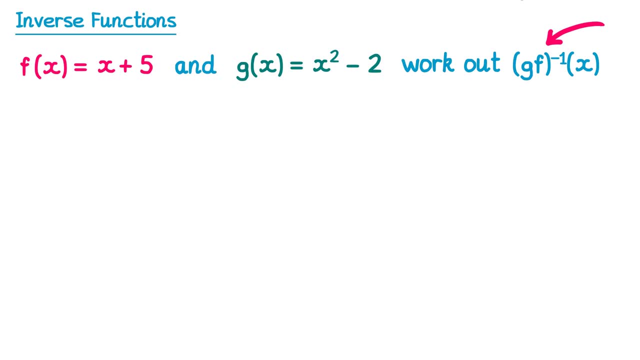 function. So we're going to start by finding the composite function g, f of x. first. To do this, we write out the g function. but everywhere we find an x, we're going to find the g function. So we're going to write brackets. So instead of x squared we write bracket squared and then minus 2.. Then 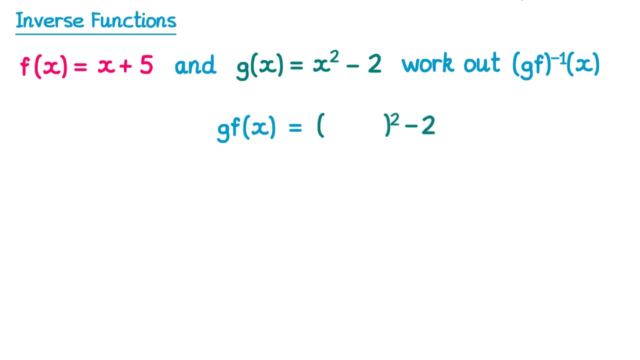 inside these brackets we write the whole of the f function. So we're going to place x plus 5 in here and that's your function g, f of x. It might be tempting at this point to expand out this bracket, but it's actually much easier if we just leave it in this form. So we're now going to find the 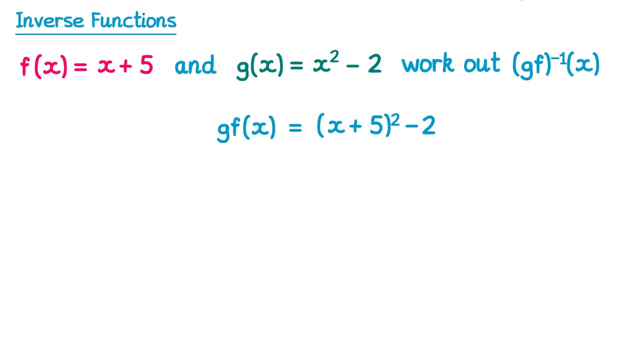 inverse of this function. So we do this in the same way we have all throughout this video. We start by replacing the function with y, So it's y equals x plus 5, all the way up to x plus 5.. squared minus 2.. Then we switch y's for x's and x's for y's, and then we rearrange to make y the.